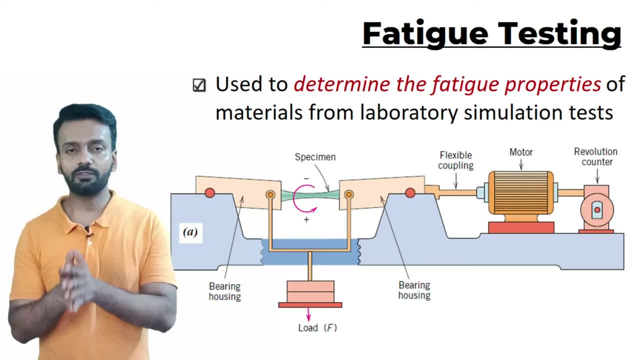 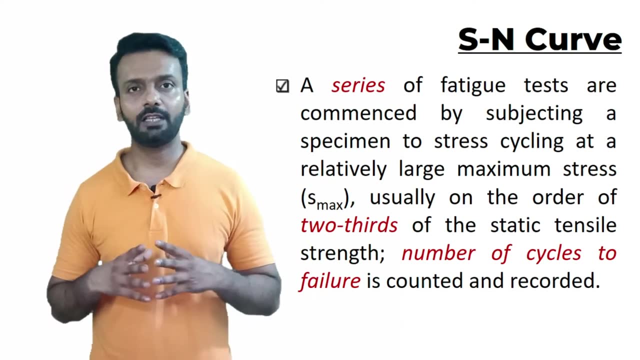 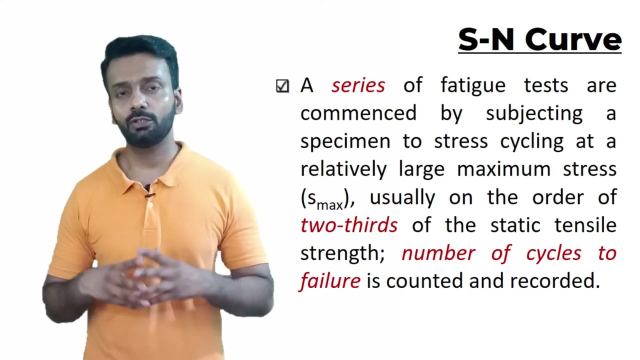 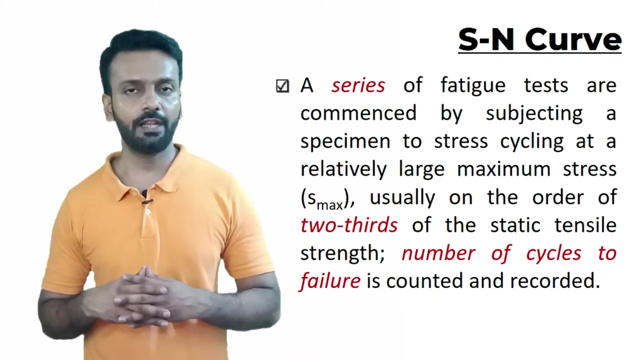 the material will fail. So we know the number of cycles to failure and that is called as a fatigue limit of the material. and this is done by this equipment which is there for fatigue testing. So a series of fatigue tests are conducted by subject of the material. then this material goes down to the cycle phase and there are series of 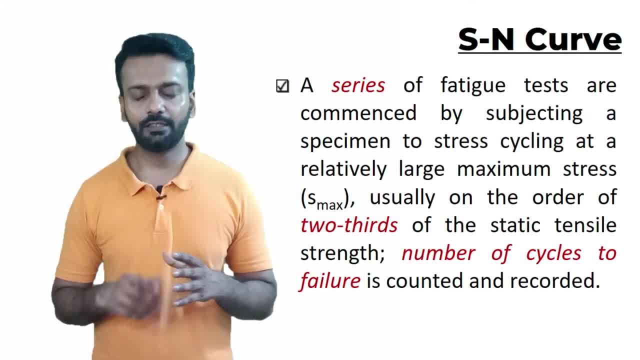 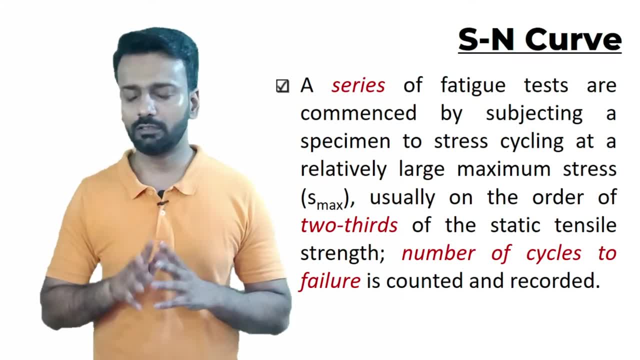 cycle phases for the failure cycle. So they are accepting a specimen to stress: cycling at a relatively large maximum stress, that is, S max, usually on the order of two third of the static, the material as they are loading and unloading the material they are counting. 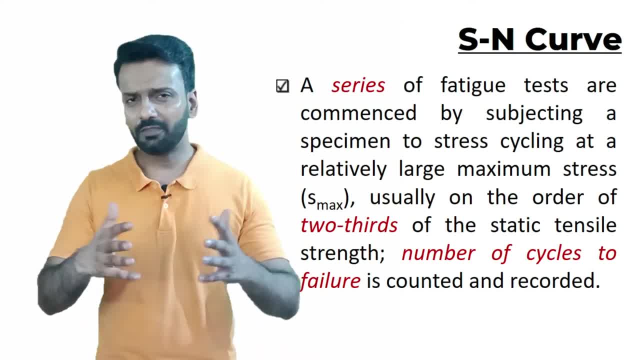 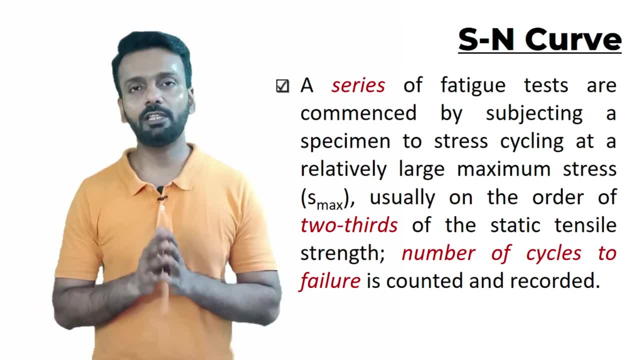 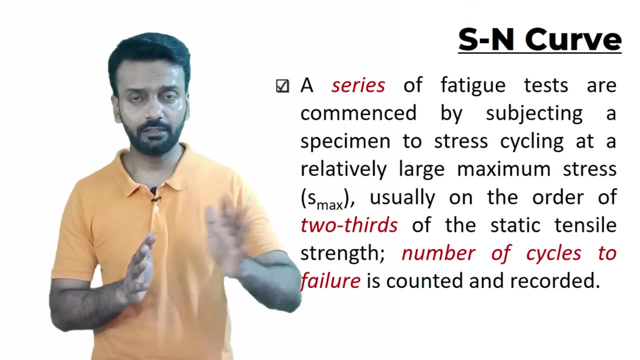 how many times they are loaded and unloaded the material and after some number of cycles, obviously the material will fail. then they will note that number of cycles. similarly, what they will do is that they will repeat these testing at a relatively lower stress than that was applied in the first. 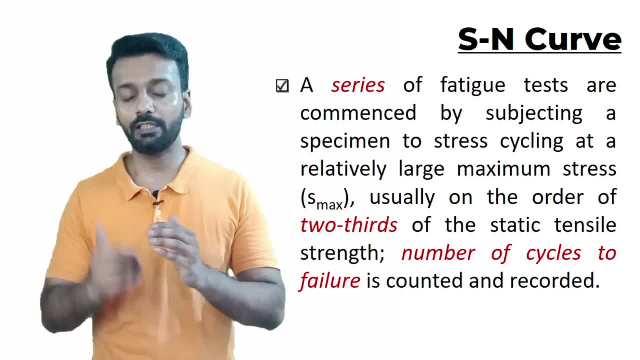 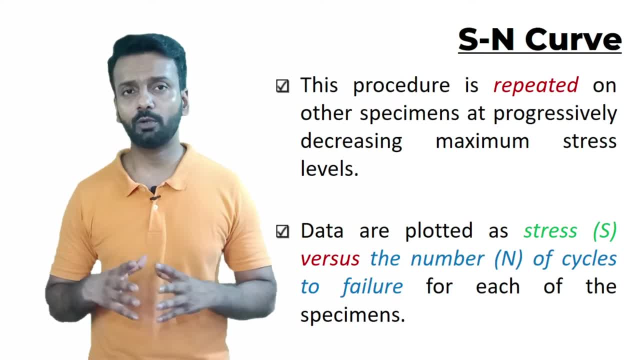 instance like that, they will keep on reducing the load and they will count the number of cycles to failure. so this procedure is repeated on other specimens: that progressively decreasing maximum stress level data is plotted as stress versus number of cycles to failure for each of these specimen. and 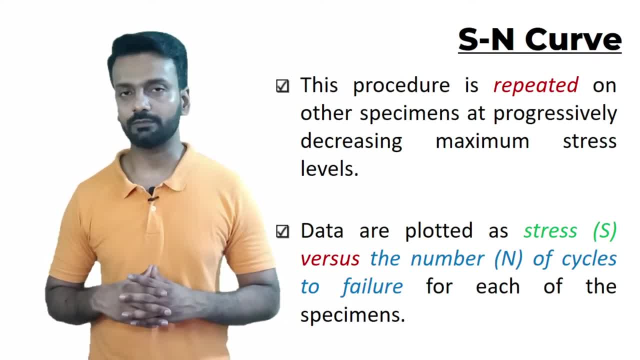 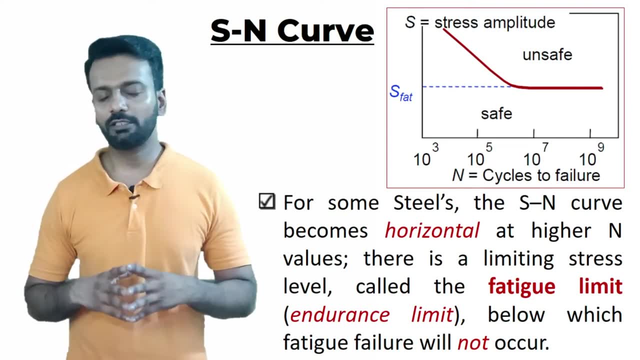 a curve is plotted, which is known as SN curve. so this is a typical lesson curve for steel. here we see the stress versus number of cycles to failure and in some steels we can see the number of cycles to failure. and in some steels we can see: 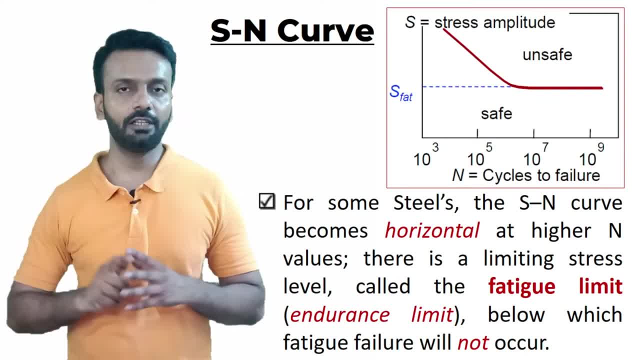 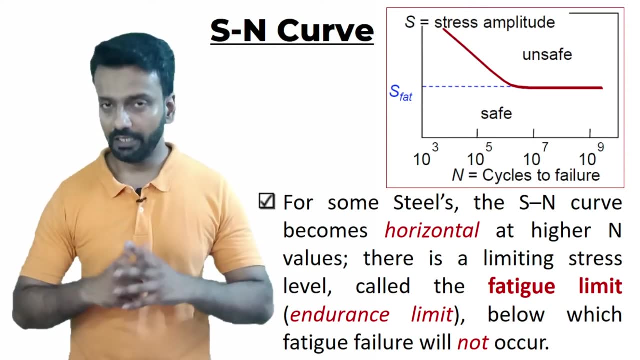 see that it comes to a horizontal line after some n number of cycles. so what does that mean is that when you apply a certain load which is well below the load of failure, the material will not fail in fatigue. it will go on and on for infinity. that is the meaning of that. so if you 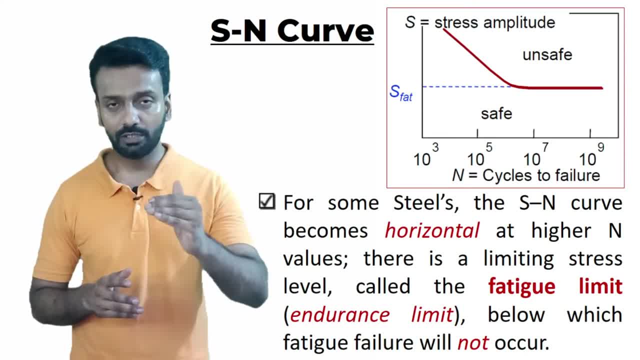 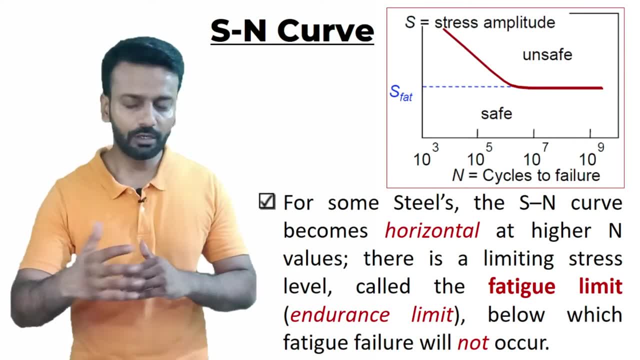 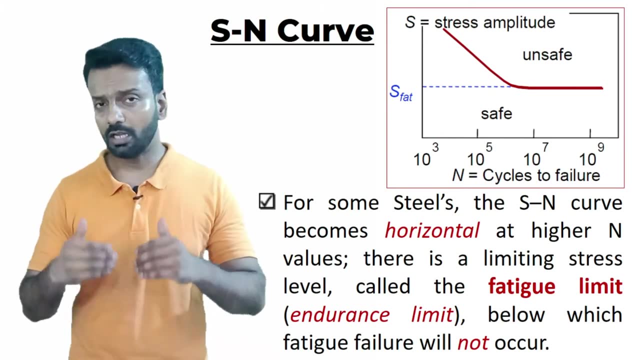 operate the material below this zone or below this level of stress, it is in the safe zone. the material will not fail. but as soon as you go beyond that stress, then the material is in the unsafe zone. and after that many number of cycles or after applying that much of load, the material will. 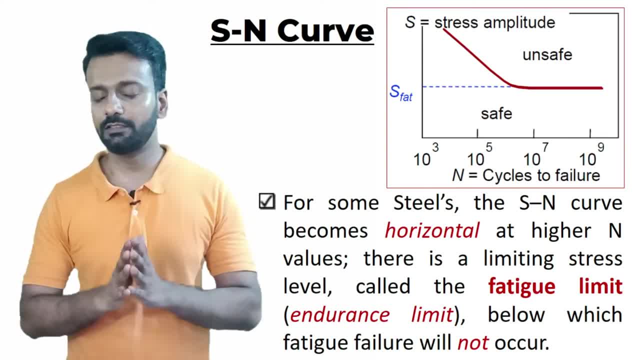 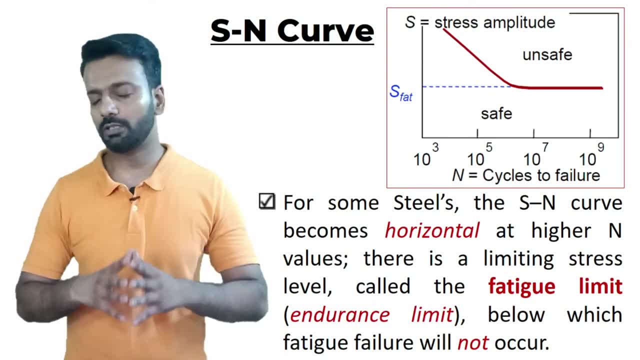 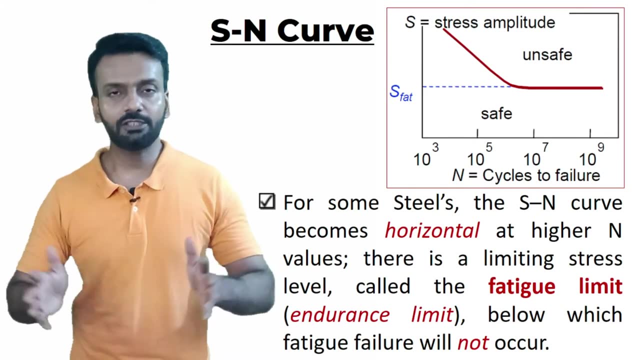 definitely fail. so for each and every material, this sn curve is defined and you know that after the material has been loaded and unloaded to these many number of cycles, it is bound to fail. so we know that when the limit of the number of cycle is approaching, we can change the component, or we can replace the component so that the 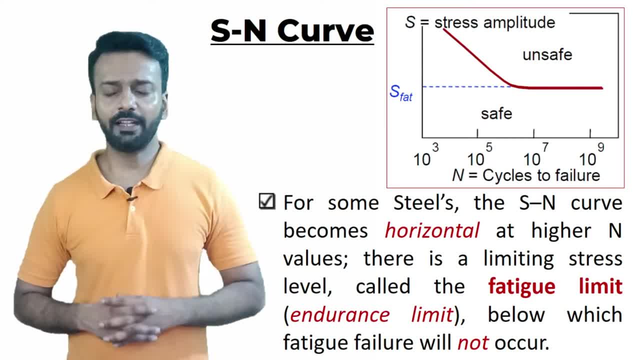 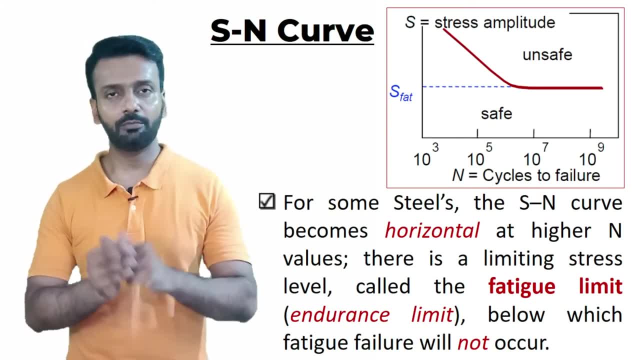 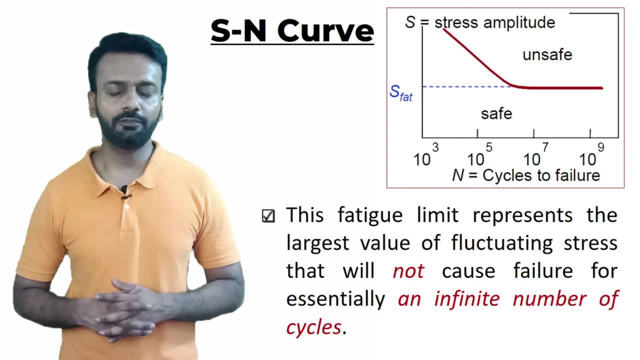 material does not fail in fatigue. so this red line which is shown here in the image is called as a fatigue limit or the endurance limit. so when you operate the material below that stress level, the material will not fail in fatigue, so mainly it will go on for infinite number of cycles. 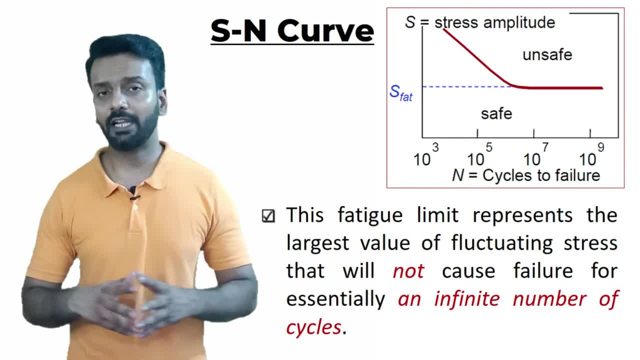 plus, whatever type of stress you apply, whether it is random stress or whether it is unilateral stress or whatever stress it may be, any fluctuating stress, the material will not fail. when you apply the load on the material which is well below the fatigue limit, it will go on for infinity and it. 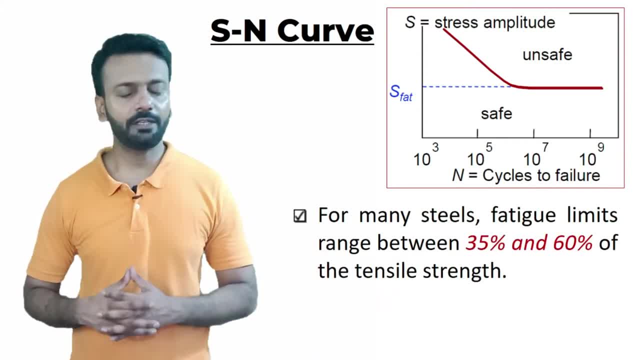 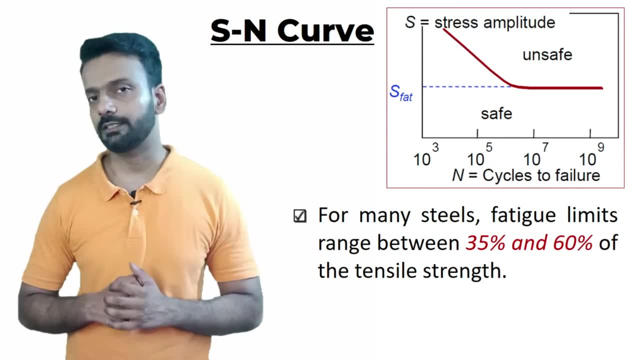 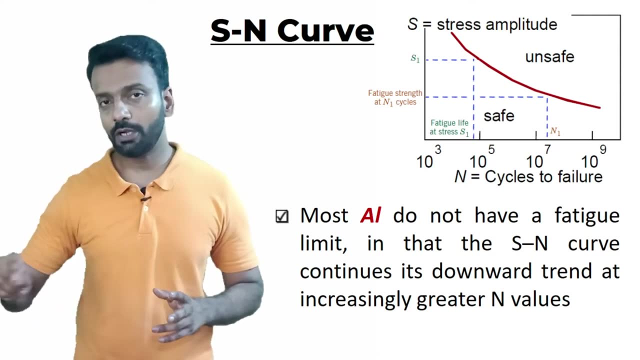 will not fail in fatigue. for many steels the fatigue limit is approximately in the range of 35 to 60 percent of the tensile strength of the material. most of the aluminum they do not have a. rather, the SN curve will go on dipping as the number of cycles they increase. so 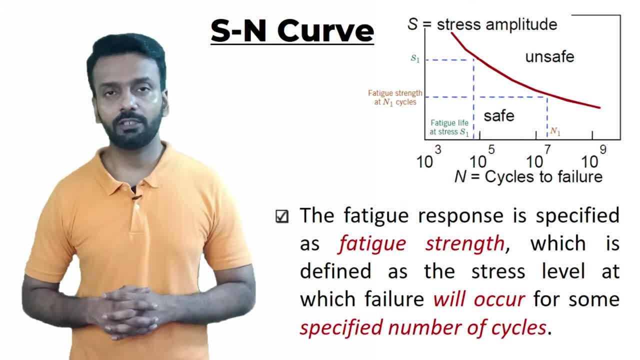 here for such type of material we have to give the failure in terms of number of cycles. so here we can't give a fatigue limit, that you operate the material to this level and it will not fail. no, that is not the case here. here we should say that after so many number of cycles the material will fail. so 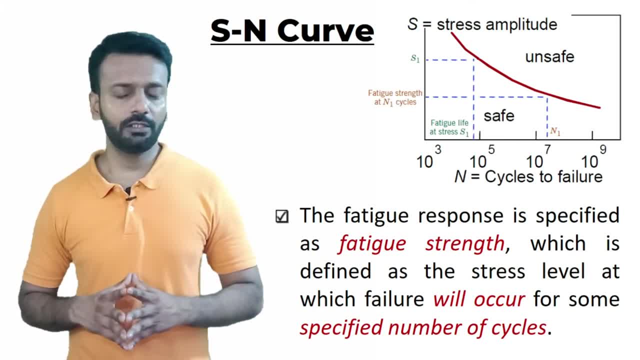 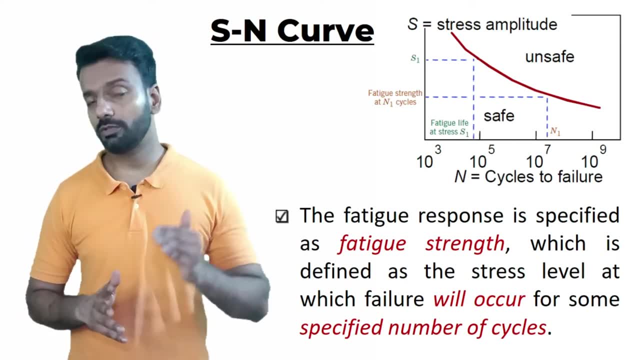 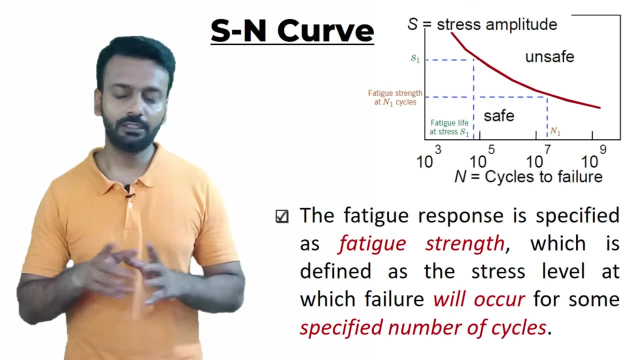 depending on what type of SN curve is there. so either you can give the failure of the material by fatigue, in terms of the fatigue limit or the endurance limit, or you can give the failure of the material in terms of number of cycles where the SN curve is decreasing throughout. so in such cases it is called 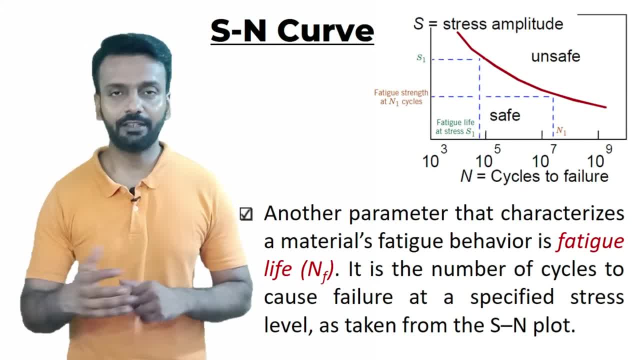 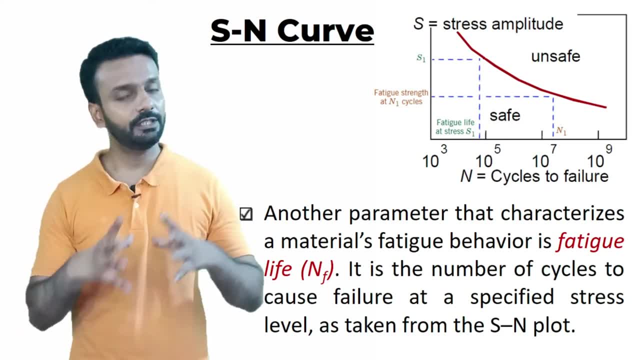 as the fatigue life of the material. that means we are telling that after 10,000 cycles the material will fail and that is the fatigue life. so it is fatigue limit or it is fatigue life. fatigue life is given in terms of number of cycles to failure. fatigue limit is given in terms 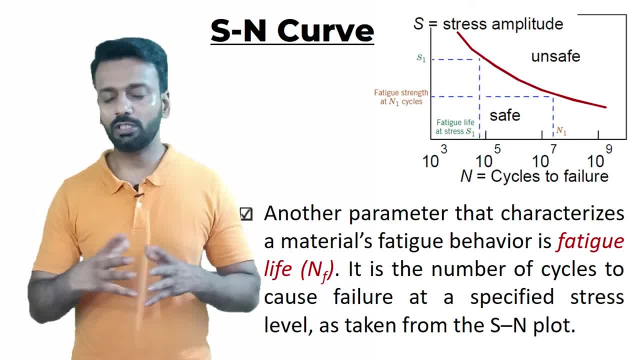 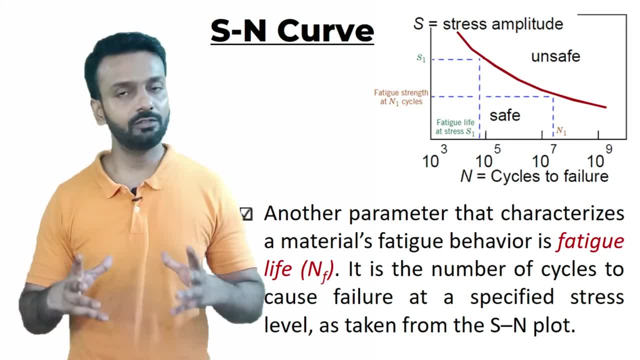 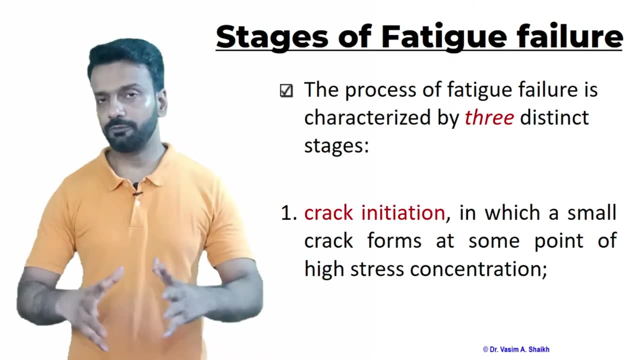 of the stress which is applied on the material and in both the cases we can say that the material is either in the safe or unsafe zone. that is how we can design the material and we can prevent the material from failure. let us see what are the different stages of fatigue failure. so the first stage is the 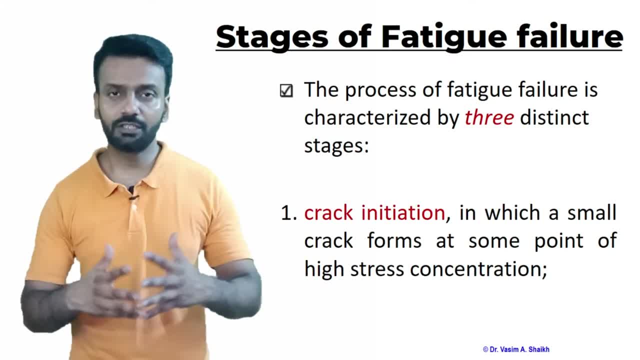 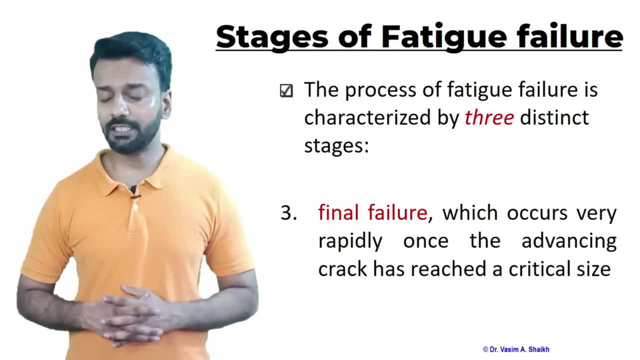 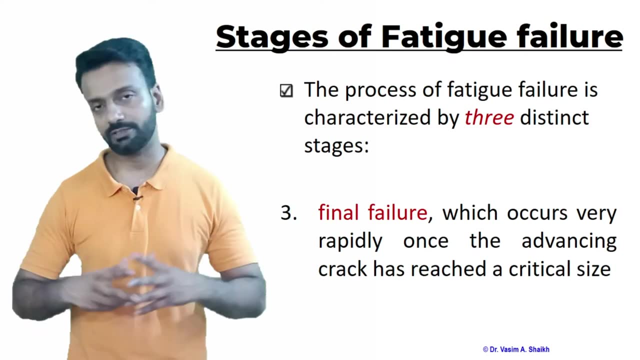 crack initiation. so here the crack starts to form in the material. the second stage is crack propagation, that means that crack is propagating. and the third stage is final rupture or final fracture, where the material basically fails and it becomes two pieces. so the first stage, that is, crack initiation, is 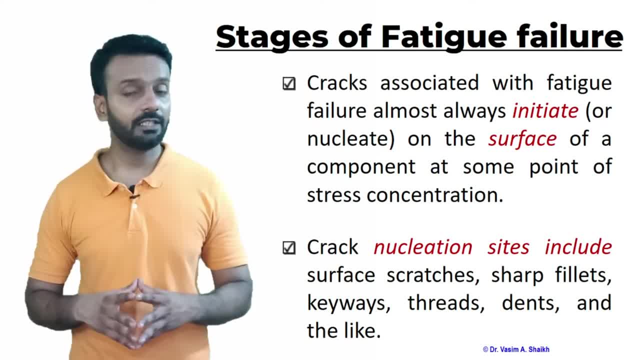 almost always formed at a place where there are stress concentrator in the material. so these concentration of stresses are to happen at a places where there are sharp corners, keyways or some impurity atoms are there or there are some dents in the material scratches. so these all 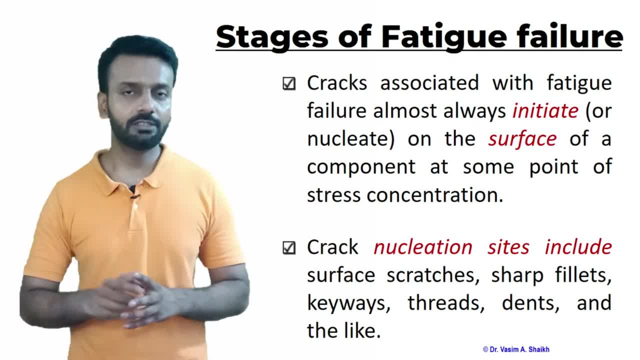 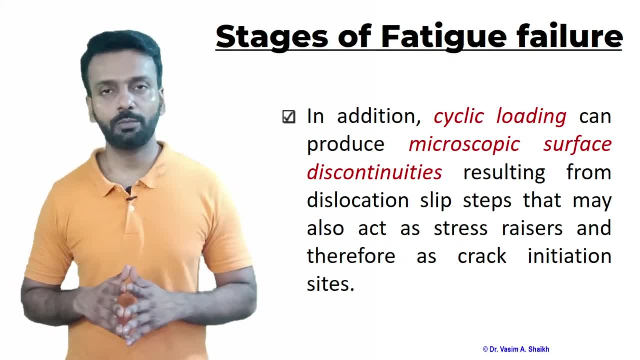 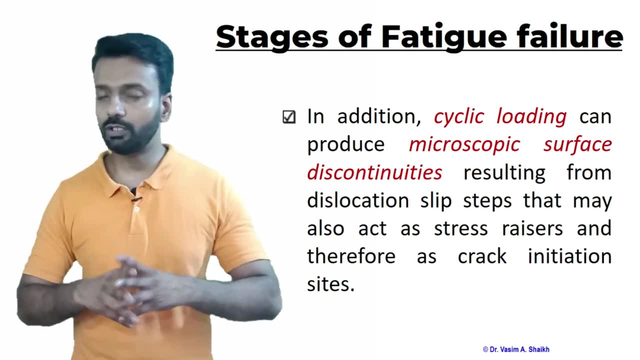 these points are the stress concentrator. always the crack will initiate from these stress concentrator. also, the cyclic loading and unloading of the material will result in some microscopic surface discontinuity internally in the material because of the movement of dislocation. this will also form the 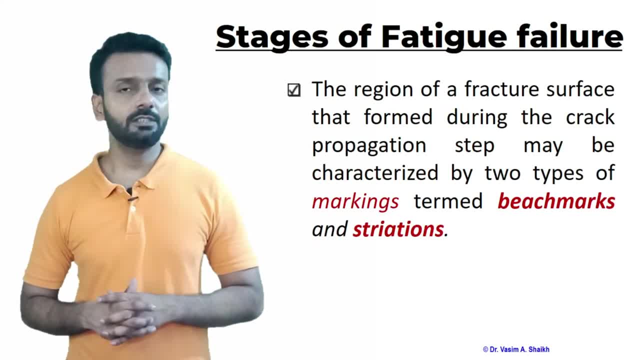 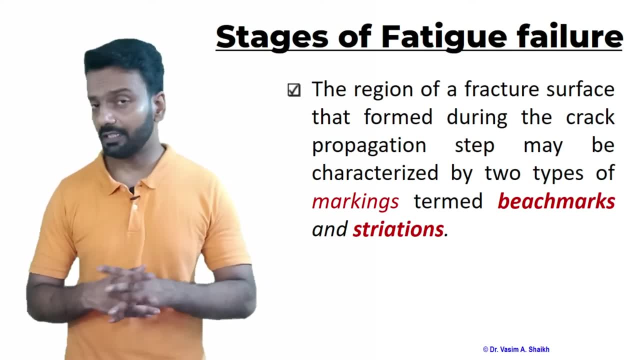 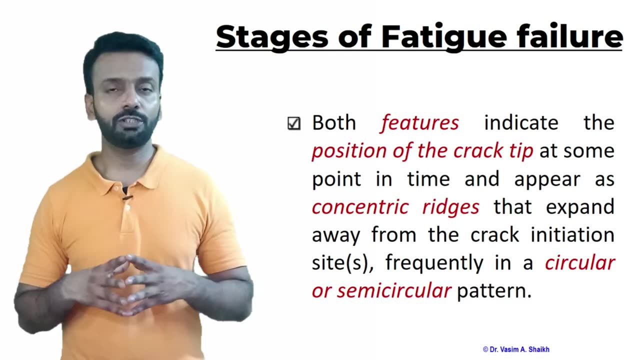 crack initiation site. next step is the crack propagation, and crack propagation can be determined in terms of two process or two things, or two markings that are happening, which are known as beach marks or striation. both these feature will indicate the position of the crack tip and the formation of the 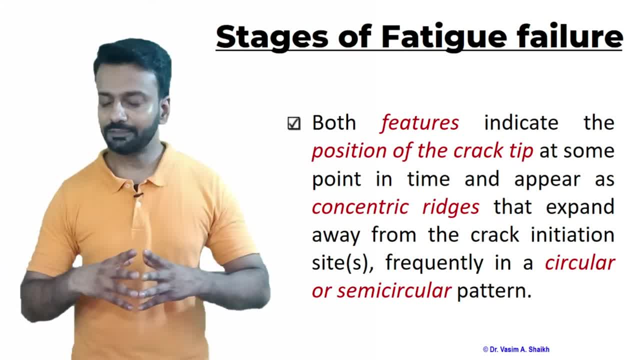 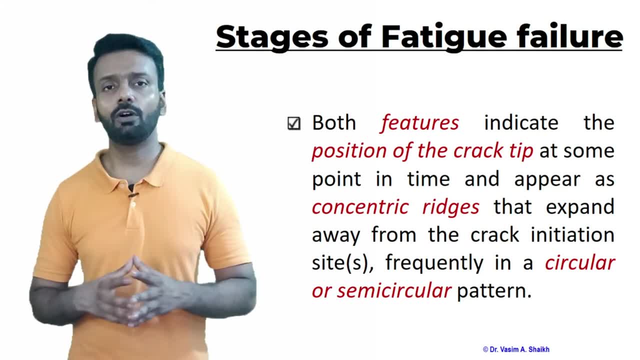 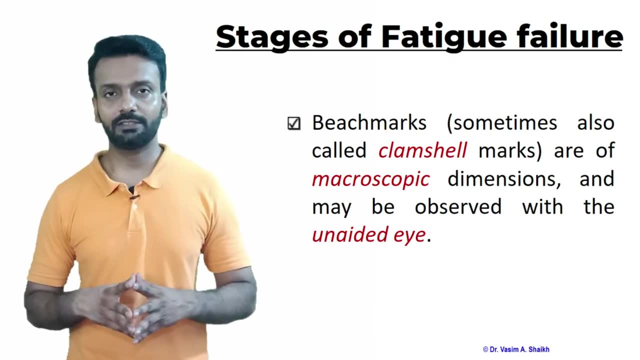 crack. also, it will tell where the crack has been initiated and where the crack has been initiated at what place, and it is determined in terms of the concentric ridges, or they are shown in terms of a circular or semicircular pattern, beach marks, also known as clamshells. they are these markings which you can see after the 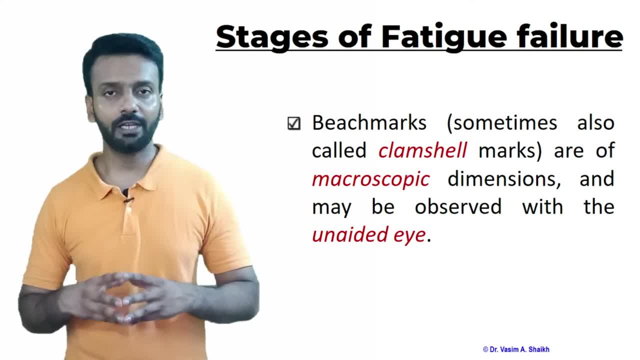 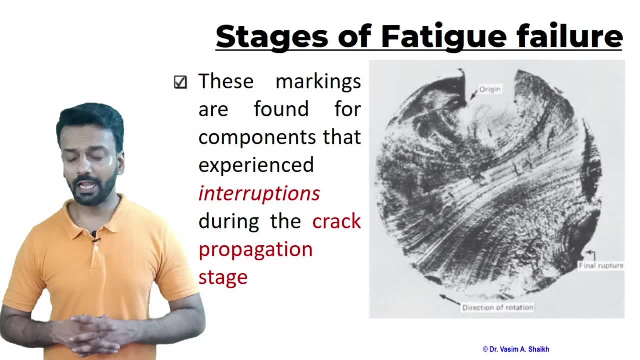 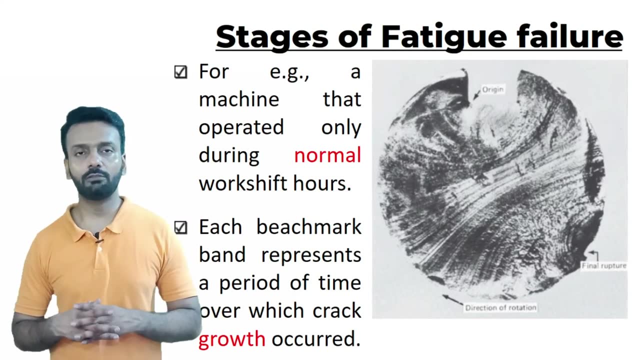 material has failed and you can easily observe them by the naked eye. these markings are formed when the material has been interrupted during the crack propagation process. as an example, we can see that when the material is propagated when the machine is operated in the normal working hour, the crack is propagating. 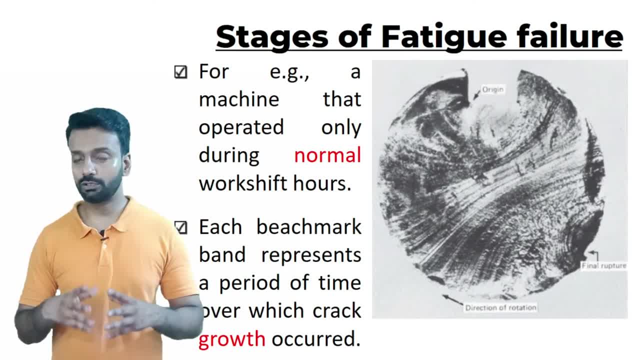 after an eight hour shift or 10 hour shift. when the machine is stopped, the crack propagation will also stop and this will appear as a clamshell marking or beach marks on the final rupture of the material. each beach mark will show the propagation of the crack during that period. 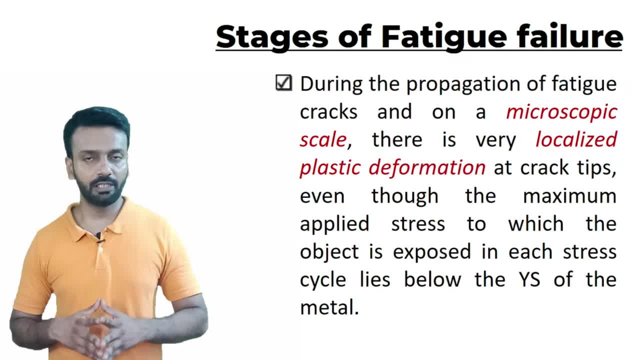 during the crack propagation stage, at a very microscopic level, there is some plastic deformation that is happening. this plastic deformation happens at a much lower yield strength of the material. this localized plastic deformation happens at a stress which is well below the yield strength of the material. this applied stress is amplified at the crack tip to the 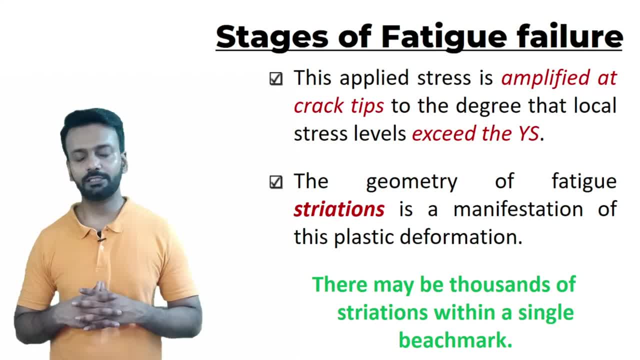 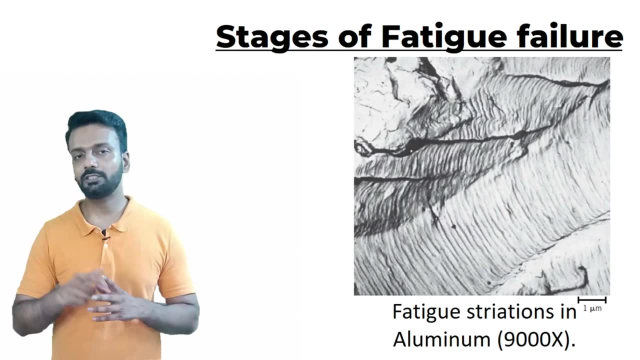 degree that local stress levels exceed the yield strength. the geometry of fatigue striation is a manifestation of the plastic deformation. there may be thousands of striations within a single day. Here we can see in this image the small, small ridges or lines which are there. these are: 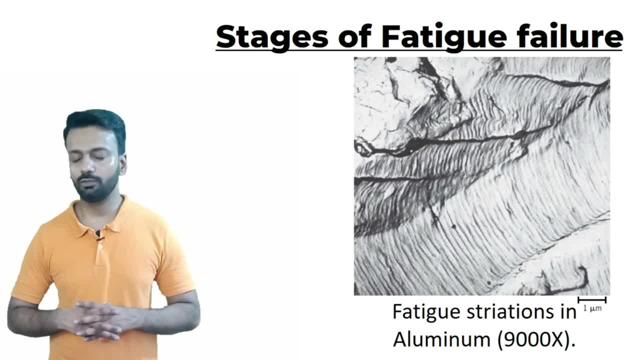 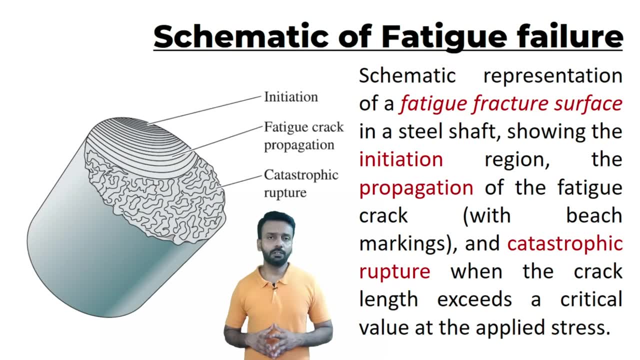 nothing but fatigue striations, which is there in this aluminum component at a very high magnification rate, that is around 9000x. let us look into this schematic of the fatigue fracture. here we can see a schematic of a shaft where we can easily locate the initiation. 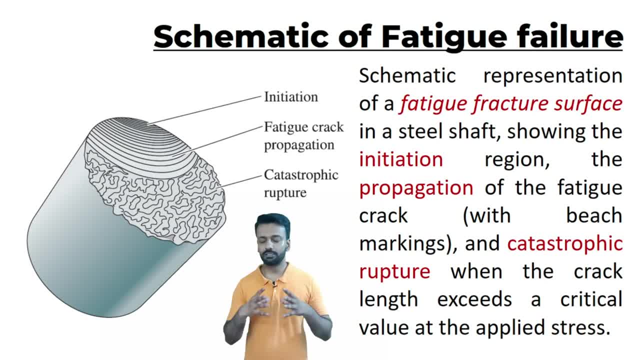 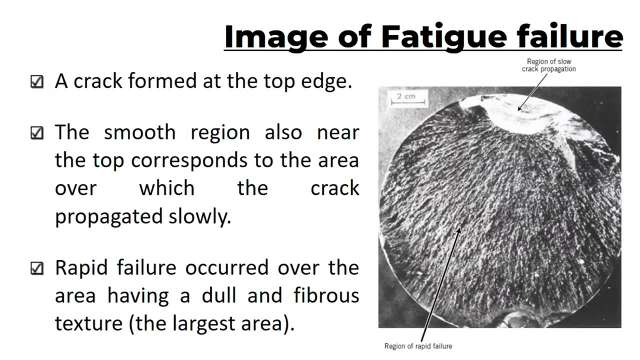 of the crack, then the propagation of the crack in terms of the striations and beachmark, and then the final rupture of the material, which shows a catastrophic failure of the material and the material has failed. this is an actual image of the fatigue failure. here you can. 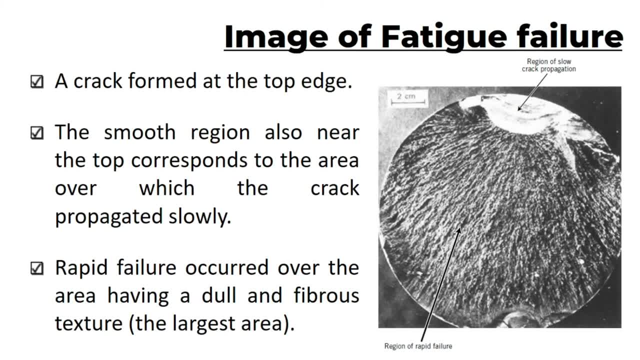 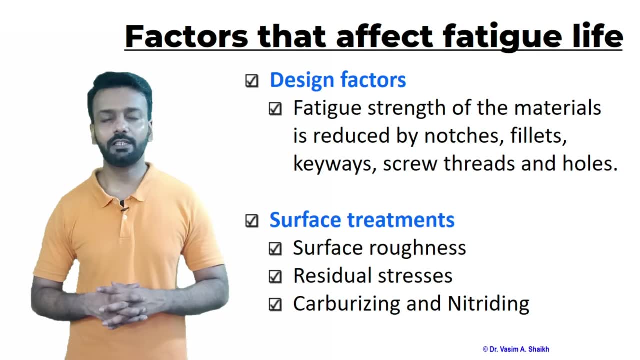 see again. we can easily locate the crack initiation, then some beach mark and then a very huge area which shows the catastrophic failure or the final rupture of the material. so what are the factors that affect the fatigue life of the material? so there are mainly two factors: design factor and surface factor. 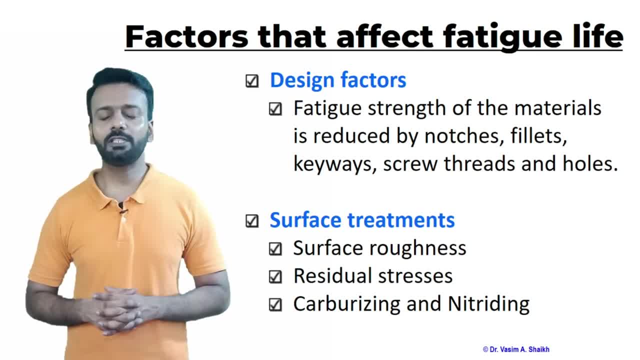 Design factor means you should not design a material where there are some abrupt changes or where there are some sharp corners, keyways and so on. Surface treatment. surface treatment means you need to design a material for proper surface roughness. when you are machining the material, the surface finish should be proper. it should